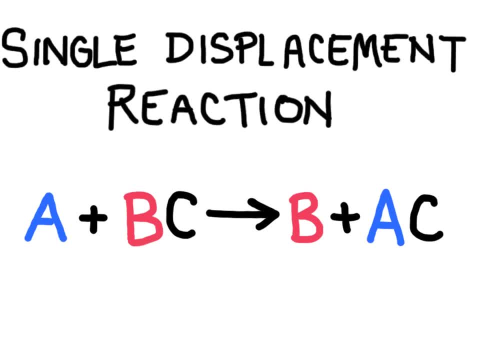 all alone is going to bump out one of the elements here of this compound, and that's what we see now. The B is all by itself and the A is joined up with this compound over here. Usually, what's going to happen is we're going to have a metal, represented here by A, that's going to swap places with 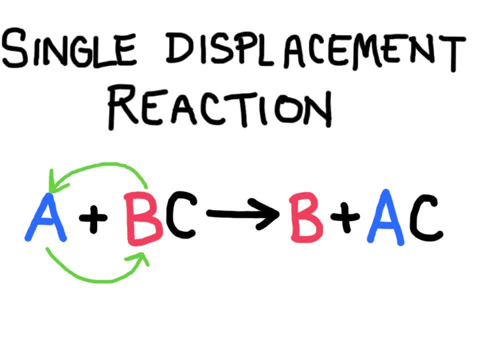 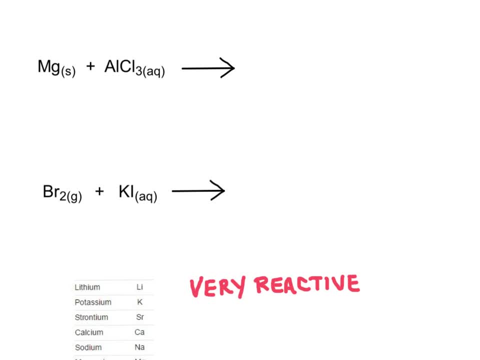 another metal that's already in a compound. So let's look at a couple examples and see how can we predict what the products are going to look like. So here's the two that we're going to look at. The first one here has magnesium. That's all by itself. here It's going to react. 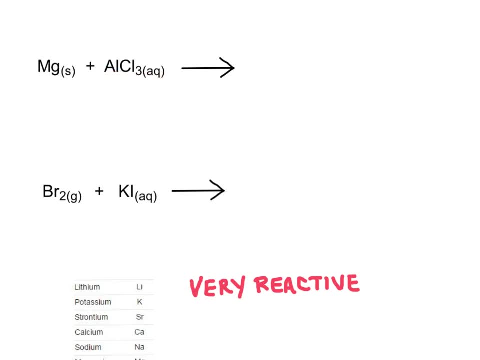 with aluminum chloride, which is represented right here. Now, these little symbols, these letters, represent the state, and so the S here means solid, and then the AQ means that it's dissolved in water, and so this stuff here would be actually dissolved in water, kind of like when you put salt table. 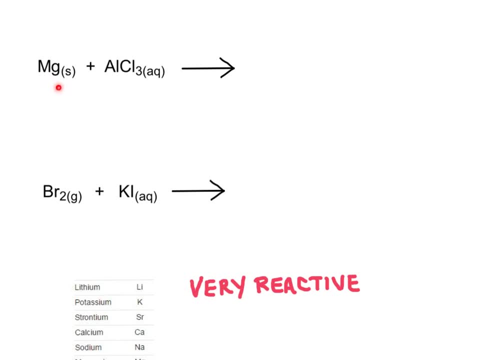 salt into water and dissolve it. Now not every single displacement reaction is going to occur, so magnesium may not be able to switch places with aluminum. It may not be reactive enough, so we think of aluminum is already reacted with chloride. Magnesium needs to be more reactive. 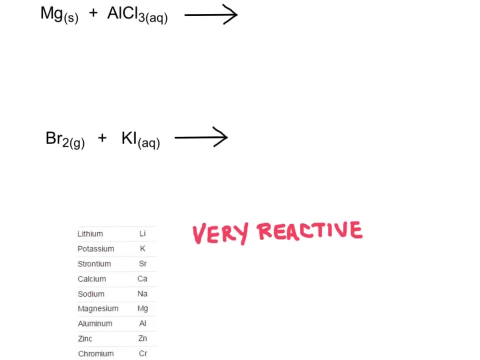 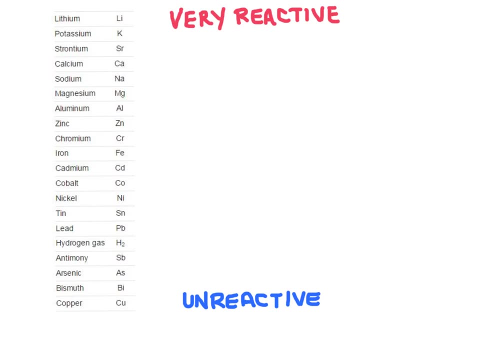 than aluminum in order to bump aluminum out of that compound. So we use something called an activity series of metal. So this is called the activity series and this shows in order here, from the bottom things that are unreactive moving up to very reactive metal. So all we have to do is 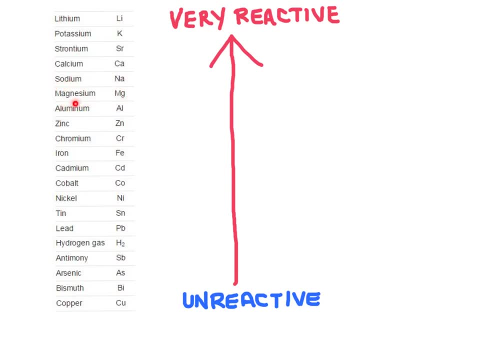 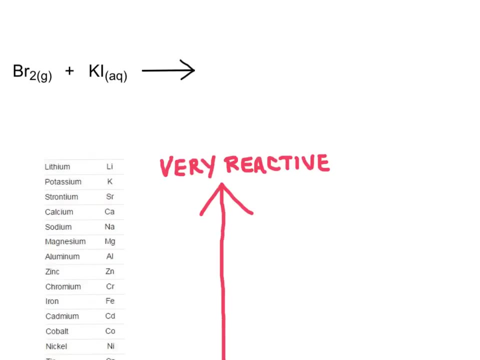 look for where's magnesium- Here it is on this list- and then look for aluminum, We can see it's going to be more reactive than aluminum, and so magnesium is just slightly more reactive than aluminum, and so that means that this top reaction here it is going to take place. So the magnesium 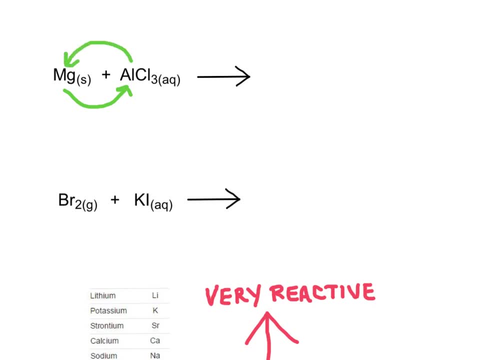 it's going to be able to bump out that aluminum. I'm going to swap places with each other and so I'm going to have. the easier part here is just writing aluminum now all by itself and put a little S to show it's solid. The tougher part here is I have to look at how is magnesium going to. 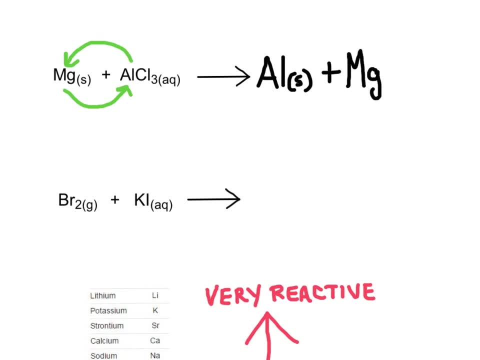 combine with the chloride. So I'm going to look at how is magnesium going to combine with the chloride? It's the Cl right here, and I have to look at the charges of these two elements because it's going to form an ionic compound. So magnesium is a metal, Chlorine is a non-metal, and so when? 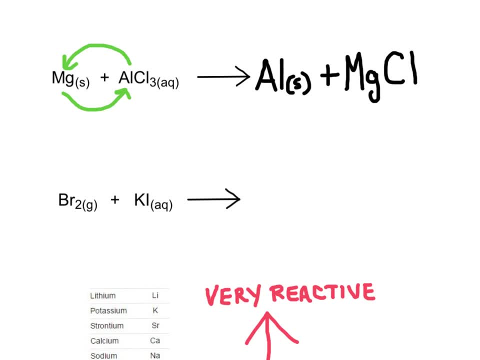 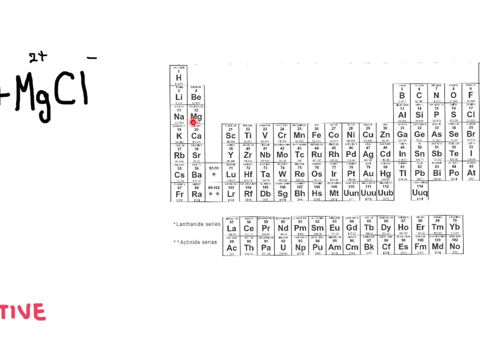 they combine together, they're going to form ions. Magnesium has a two plus charge, Chlorine has a minus one charge and I know that because of their locations on the periodic table. So I can see: here's magnesium, It's in group two. So here's group one, here's group two, Everything here has a two plus charge and 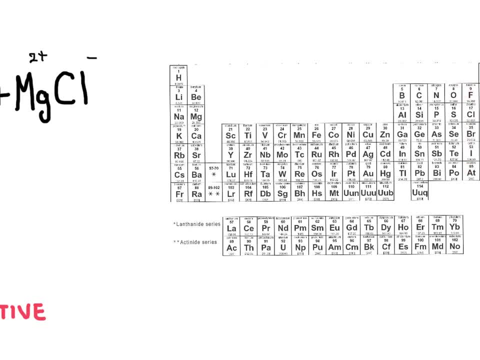 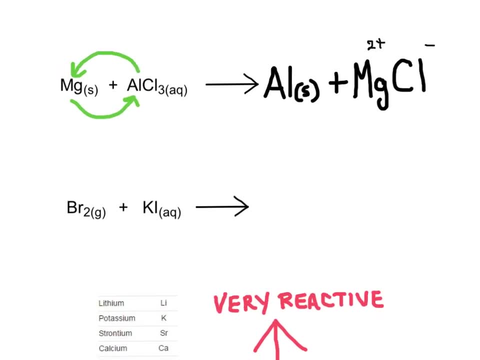 then chlorine is over here in group seven. Everything here in group seven has a minus one charge, and so I need to get those charges to balance each other. So I'll need two chlorines, and this will be dissolved in water, and so I'll just put a little AQ there to signify that. So the top one involved two metals. 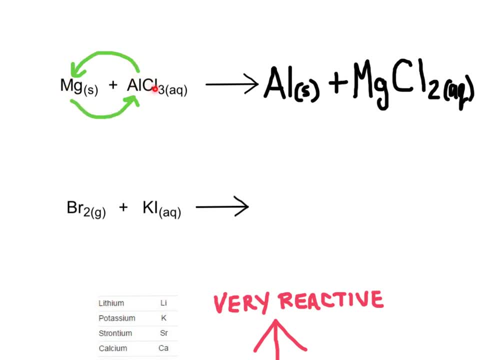 Switching places with each other. and then we had the non-metal of chlorine is going with magnesium. Down here at the next one, I have bromine, which is a non-metal. It's going to react with potassium iodide. This is an ionic compound, so we have 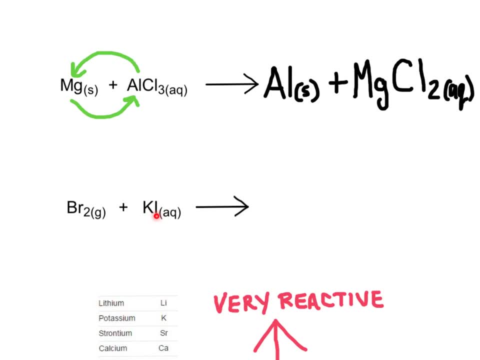 potassium is a metal and iodine is a non-metal, So there's not two metals to switch place here. In this case we're going to have the two non-metals switching places with each other, So we can either have two metal switching. 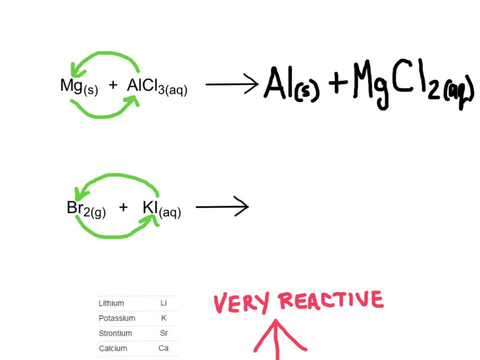 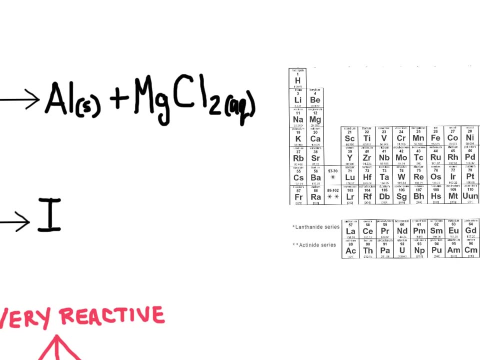 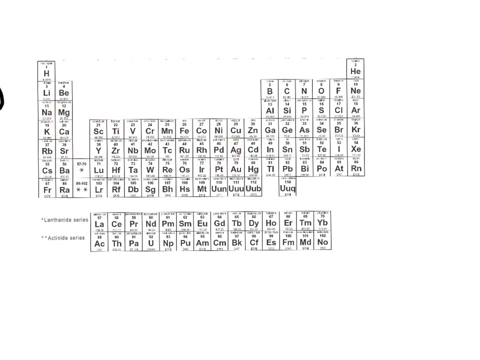 or to non-metals, switching places. So in this case, iodine is going to be all on its own, and the one thing we need to keep track of here is: what do elements look like when they're by themselves? Now, magnesium, and pretty well all metals, are just going to be the symbol, and then 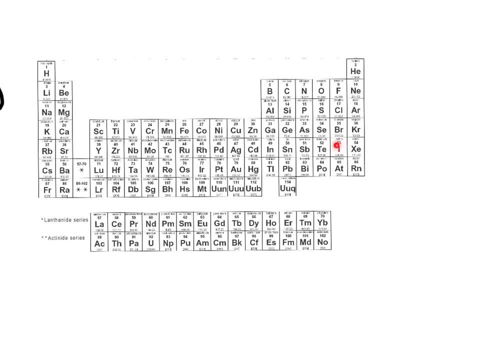 a little s to show it's solid. Iodine right here is a diatomic element. That means when it's found by itself in nature, it exists as two atoms bonded together. That means diatomic and there are seven diatomic elements: Nitrogen, oxygen, fluorine, chlorine, bromine and iodine. So these six right.